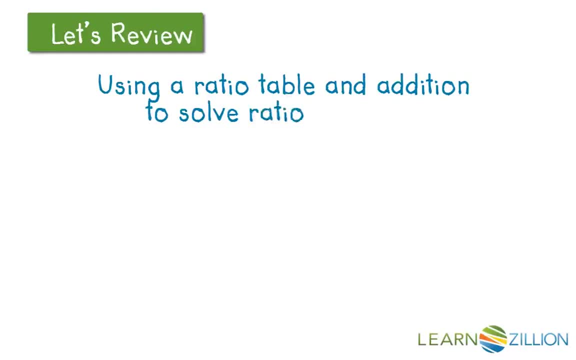 Let's review how to use a ratio table and addition to solve ratio problems. Here's what it looked like when we did that, And you can see that we used the pattern of the ratio to fill out this table, Always adding 2 cups of grape juice for every 3 cups of apple juice, until we got to 12 cups of apple juice and our answer of 8 cups of grape juice. 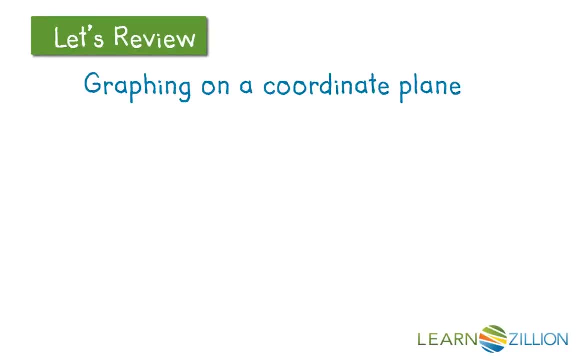 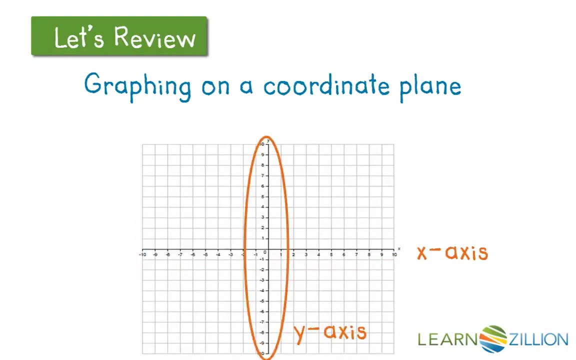 For this lesson, we also need to review how to graph on a coordinate plane. So here's a coordinate plane. Remember, the horizontal axis is the x-axis, The vertical axis is the y-axis. The point where they cross is called the origin. 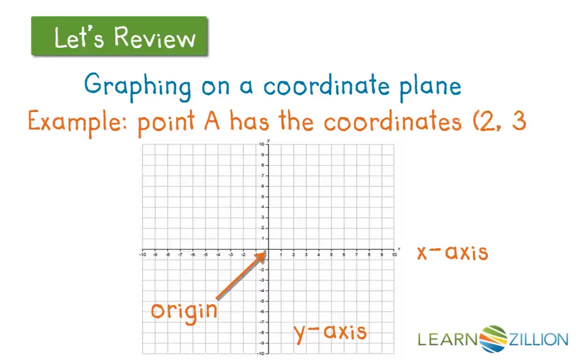 An example is: you might have to graph a point that has the coordinates. Remember, the first number is called the x-coordinate and the second number is called the y-coordinate, So that 2 we're going to graph on the x-axis by going over 2 squares to the right. 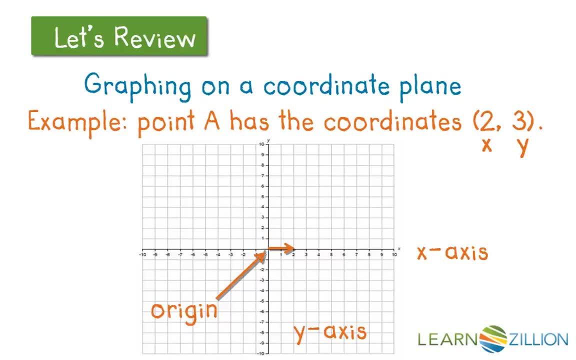 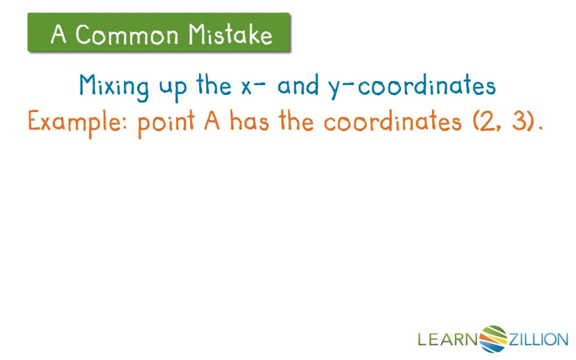 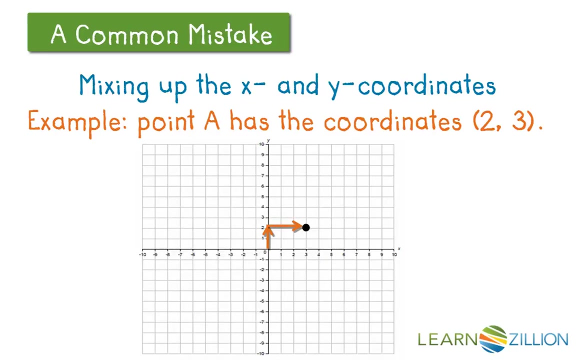 And then the 3. we'll graph on the y-axis by going up 3 squares. So point A is right here. At Sometimes students make the mistake of mixing up the x and y-coordinates. So with our example, a point that has the coordinates, a student might go up 2, then over 3 and put point A right there. 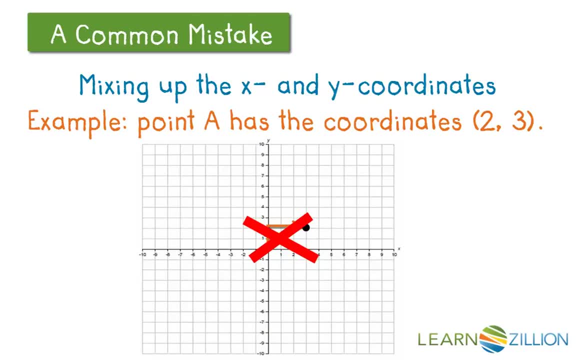 This is incorrect because the x and y-coordinates are mixed up. Always remember that the first coordinate is for x and the second coordinate is for y. x comes before y, just like in the alphabet, And then the x-coordinate goes on the horizontal x-axis and the y-coordinate goes on the vertical y-axis. 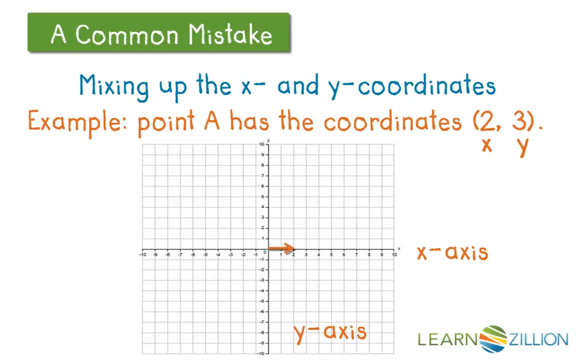 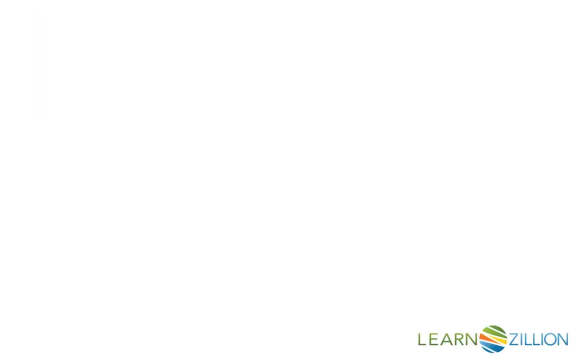 So first you need to go over 2, then on the y-axis, up 3 to correctly place point A right there. Okay, here's the example. we're working on our fruit punch example And you can see the ratio: 2 cups of grape juice for every 3 cups of apple juice. 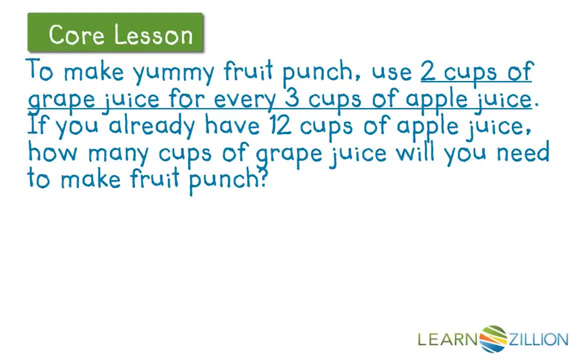 The problem also tells you that you already have 12 cups of apple juice, So we can use this information to fill out a ratio table, just like we've done before. The only difference here is that I've stuck in that first column with 0, 0, and that makes sense. 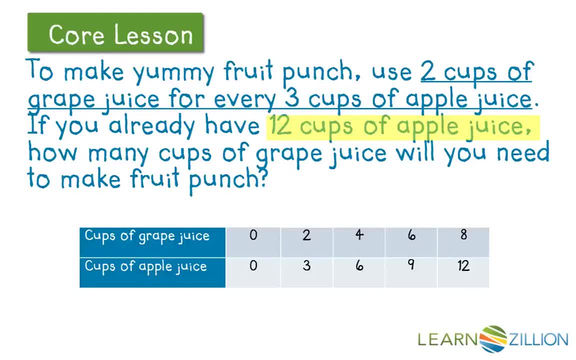 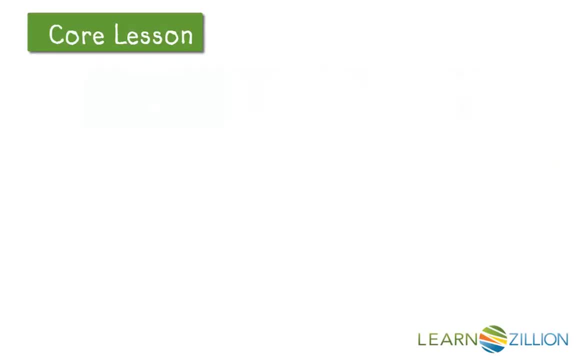 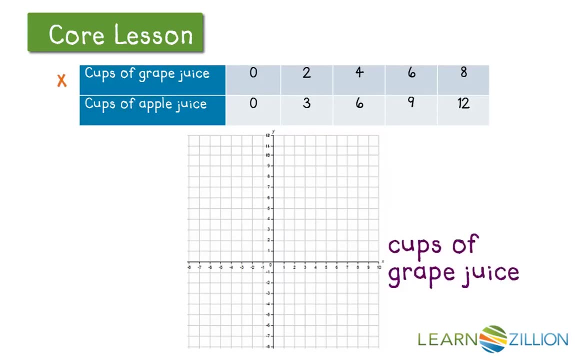 If you don't have any grape juice, you're not going to have any apple juice. We add in that column because it's going to be important for graphing. So now let's represent that ratio table on our coordinate plane. We'll call grape juice x, so that we'll be graphing cups of grape juice on the x-axis. 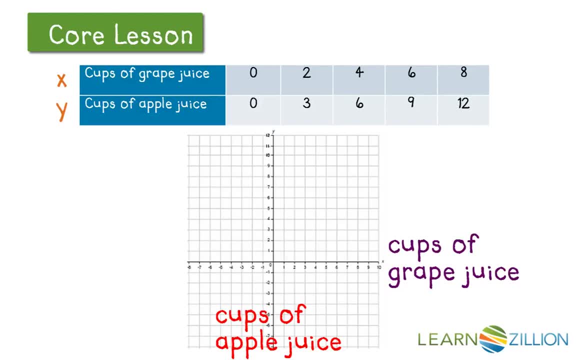 And we'll call apple juice y. so we'll be graphing apple juice on the y-axis. Our first point will come from the first column in the table: 0 cups grape juice and 0 cups apple juice on the coordinate plane. that's right there at the origin. 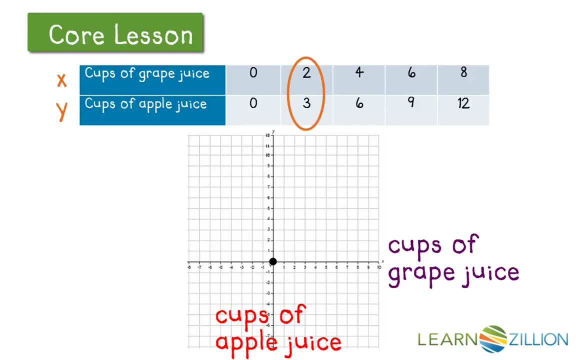 Our next point will come from the next column of the table. So we need to show 2 cups of grape juice going over 2 squares on the x-axis And 3 cups of apple juice, which will be going up 3 squares on the y-axis, to put a point right there. 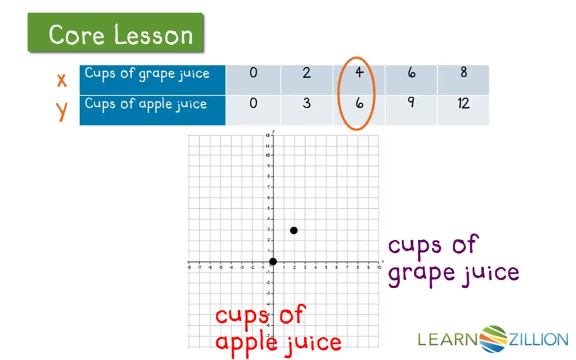 Our next point will be 4, 6.. So going over 4 on the grape juice x-axis and up 6 on the apple juice y-axis, to put a point right there, And then we'll just keep this pattern going until we get to the point where there are 12 cups of apple juice. 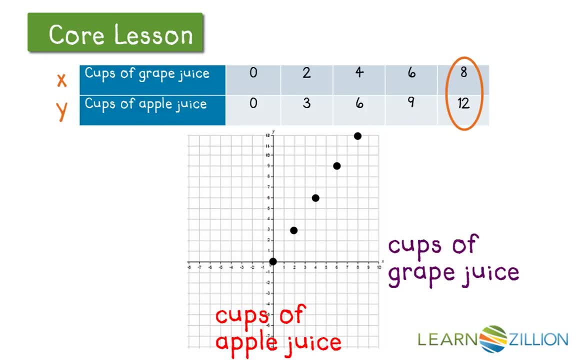 And right there, when we graph it, we can see that there will be 8 cups of grape juice. The same answer we've been getting using different methods and now just we're seeing it on a graph, a new way of doing it. The same addition relationship that we see in a ratio table, adding 2 cups grape juice for every 3 cups apple juice. 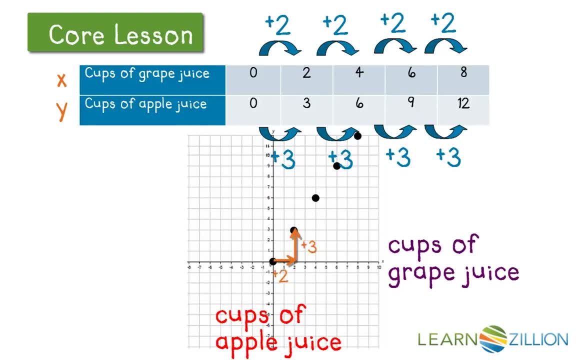 we can also see that on our graph. We're always adding 2 cups of grape juice and 3 cups of apple juice to get to the next point, Always going to the right- 2 and up 3.. Our final step here is just to draw a line to connect those points, and there you have it.